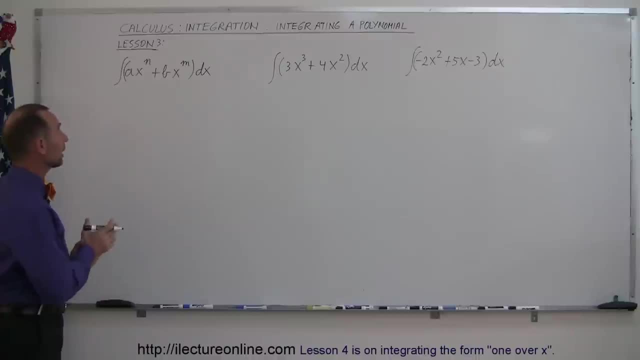 Welcome to our lecture online, and here's our third lesson in how to integrate. In this case we're going to show you how to integrate a polynomial. So here we kind of combine what we've learned in the first couple of lessons, and then there's something in addition here. So what do we do when we have, for example, two terms that are added together, forming a polynomial? Well, it turns out we can actually rewrite that as two integrals, separated like that. So ax to the n power times dx, plus the integral of bx to the n power times dx. 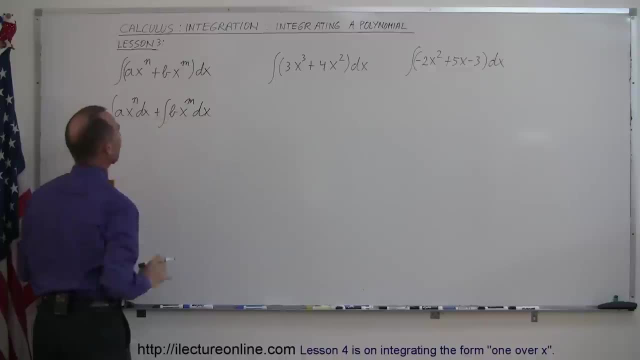 So we can actually separate each term into its own separate integral. And then, applying the rule that we learned before, we can actually take the constants- assuming a and b are constants- and move them outside integral sine. So this is equal to a times the integral of x to the n? dx plus b times the integral of x to the m dx. Notice that n and m just simply imply that they don't have to be the same number, They can be two different numbers. And now we can apply the rule that we learned before So we can actually separate each term into its own separate integral. 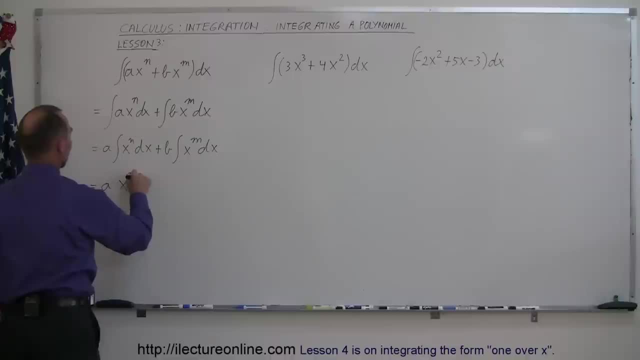 So we can say that this is equal to a times x to the n plus 1.. We add one to the exponent, divide by the new exponent, n plus 1.. And then we add a constant of integration- We'll call it c1- as a constant of integration of the first integration. And then we do the same to the second one, So plus b times x to the m plus 1.. We add one to the exponent and then divide by the new exponent, m plus 1.. And then we also add a constant of integration, We'll call it c2.. 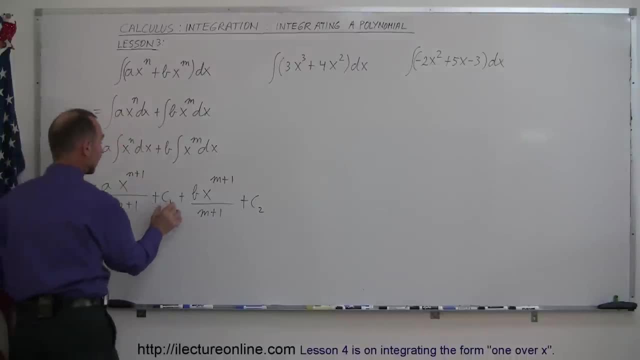 For that integral. And then you can add c1 and c2 together, because they're just any arbitrary constants. Add them together and simply say there's a constant at the end. So we can then write this as a times x to n plus 1 exponent divided by n plus 1 plus bx to the m plus 1 over the new exponent m plus 1, plus a constant of integration. And that's the integral of our polynomial, like that: 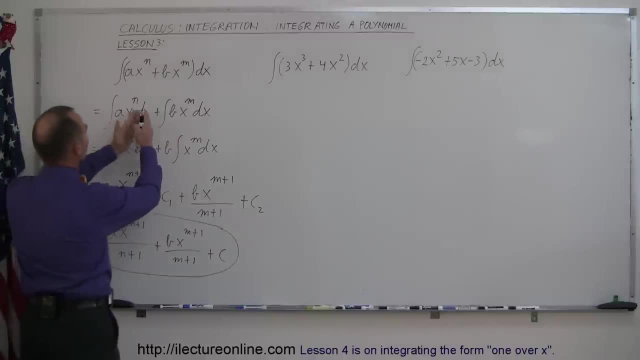 So We can see that all you can do, all you. what you can do is you can separate these, write a separate integral for each term in the polynomial, then move your constants outside an integral sign and then use the power rule here.